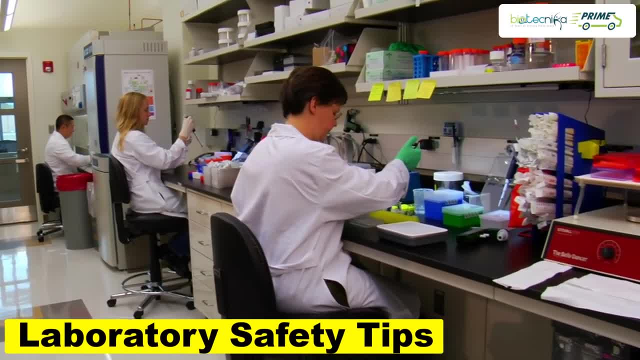 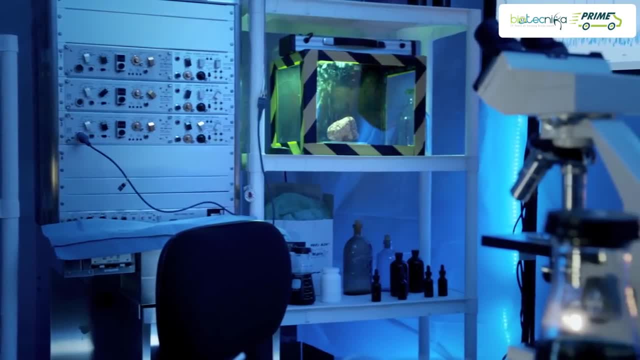 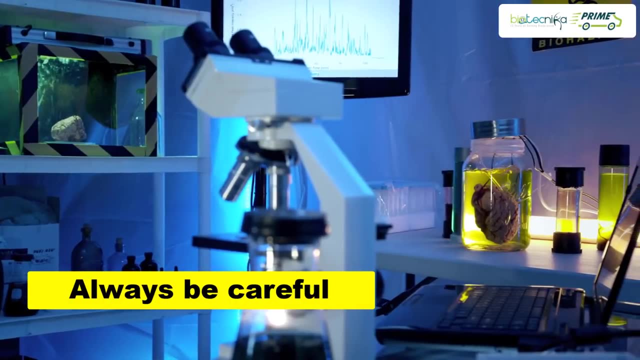 So today I took some time to remind you all about the lab safety tips which all of us often tend to miss. Laboratory safety is as simple as our alphabets A, B, C. Always be careful. Safety is important, whether it's on road, at our houses, kitchens or laboratories. 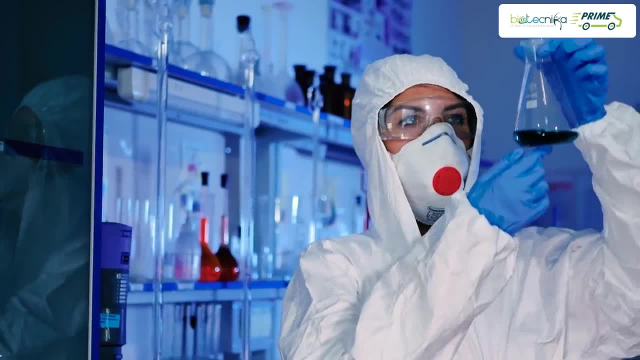 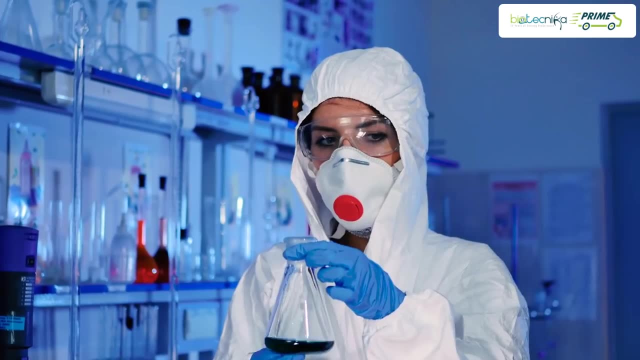 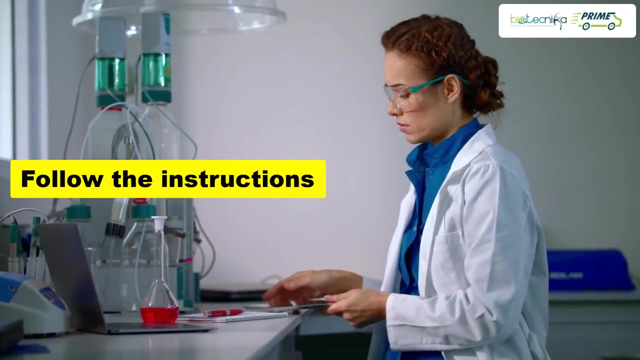 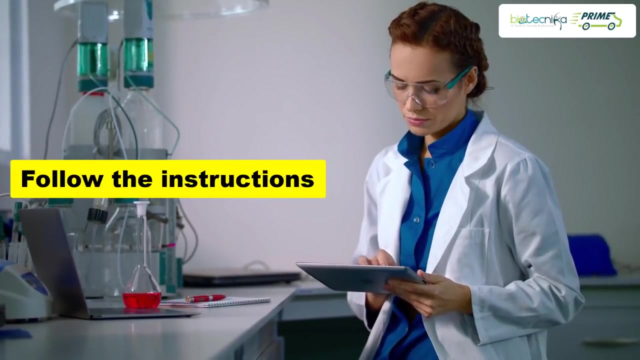 We tend to consider the safety everywhere, Then why not in our laboratories? Safety in the laboratory is the key or path to successful experimentation. Here I am enlisting the top 10 general laboratory safety tips. Number 1. Follow the Instructions. It is important to follow the instructions of the manual, guide or laboratory expert. 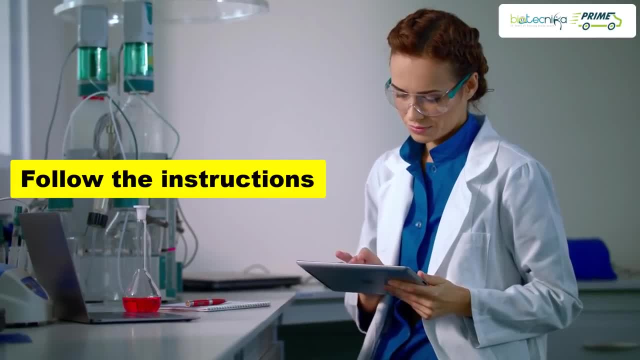 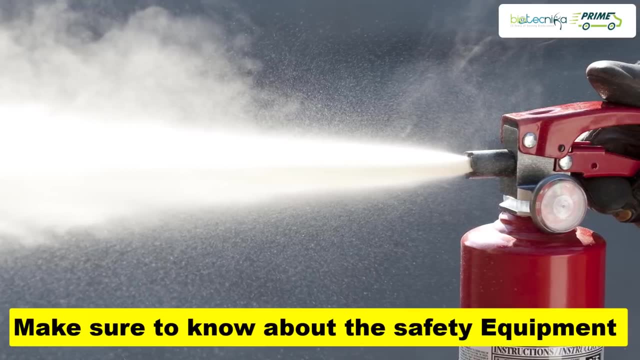 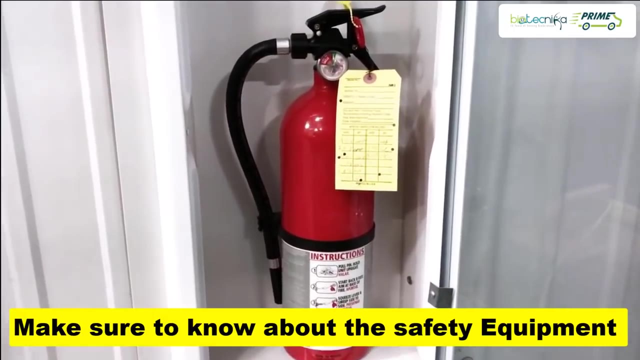 Tiny carelessness can create a mishap. Always go by the rules Number 2.. Make sure to know about the safety equipment. Always keep in mind where the safety gears and other emergency safety equipment are kept. Make a habit of checking those safety time to time in order to ensure their proper working. 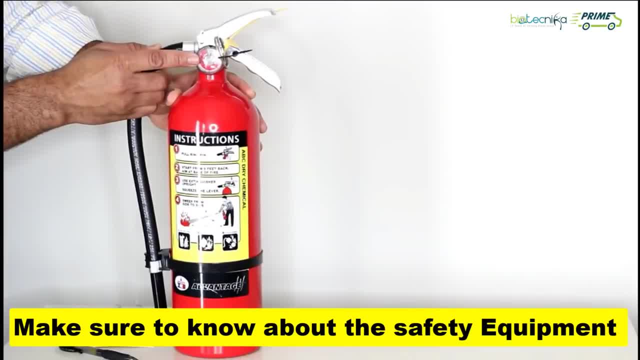 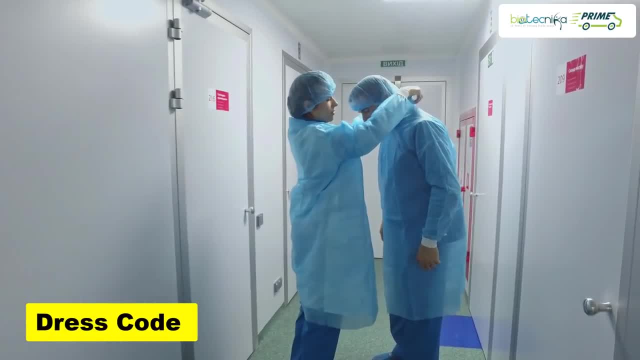 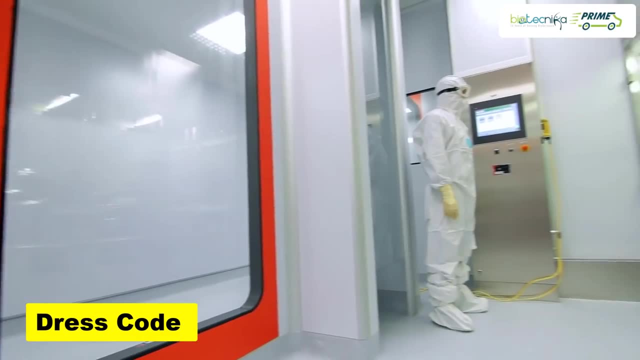 Make a well-designed budget for these requirements and also buy quality chemicals and laboratory products. Number 3. Dress code. Follow proper dress code when you are in the lab. Do not wear loose clothes. open mouth footwears must be avoided. Long hair must be tied up. 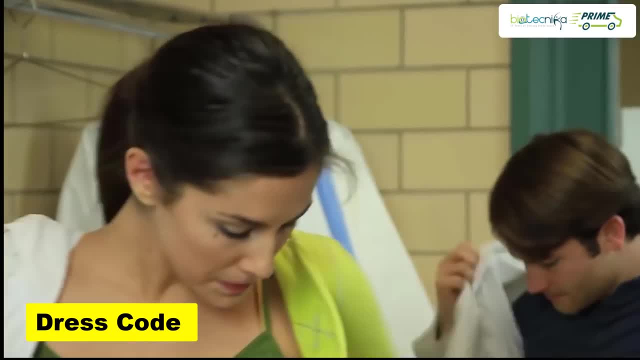 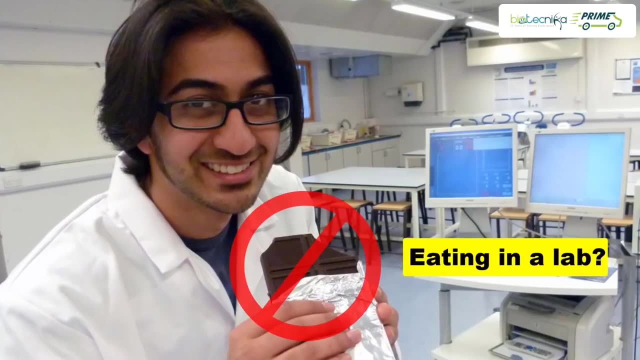 Use proper gloves, eye gears and lab aprons while working and when present in the lab Number 4.. Eating in a lab: A strict no-no. This habit will not only ruin your experiment, but also cause an adverse effect on your health. 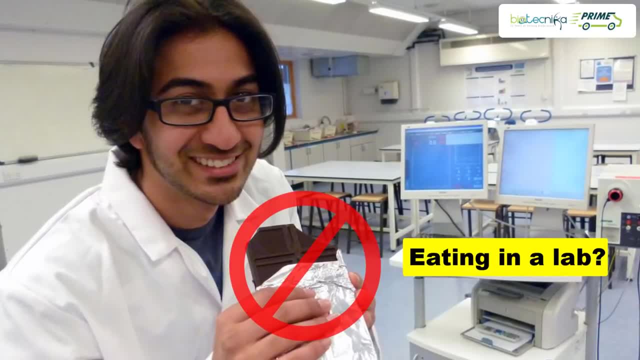 Number 5. Eating in a lab: A strict no-no. This habit will not only ruin your experiment, but also cause an adverse effect on your health. Number 5. Eating in a lab: A strict no-no. This habit will not only ruin your experiment, but also cause an adverse effect on your health. 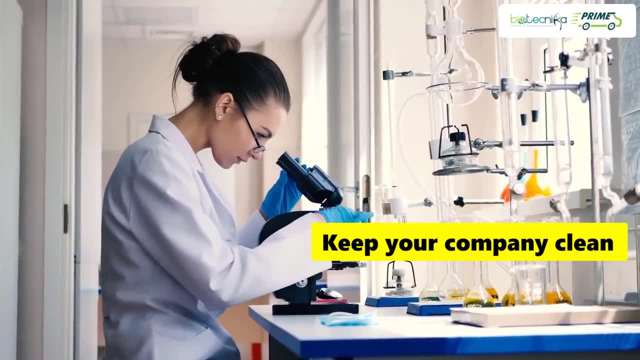 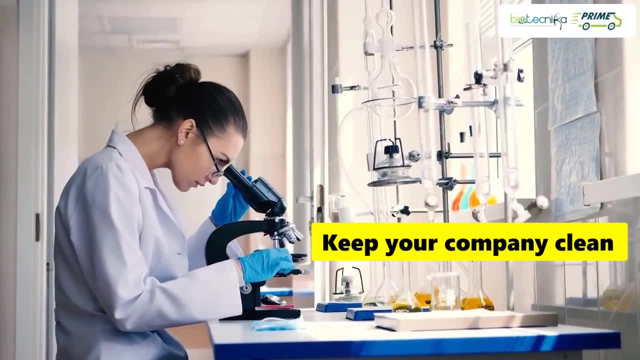 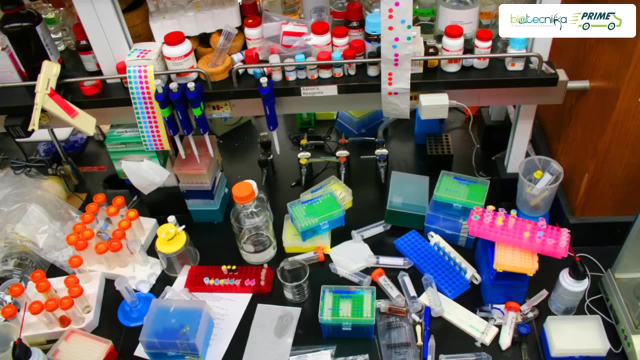 Number 5. Keep your company clean. Avoid people who tend to distract you while working with instrument and reagents. They may hamper your experimentation, causing some damage. It is advisable to act responsibly while handling any chemicals or laboratory instrument. Number 6. Clean your own mess. 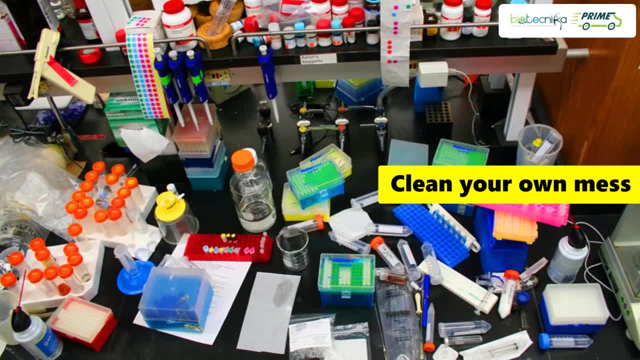 This habit is very annoying for all of us. We may have many fellow researchers who tend to start their own research. We may have many fellow researchers who tend to start their own research. We may have many fellow researchers who tend to start their own research. 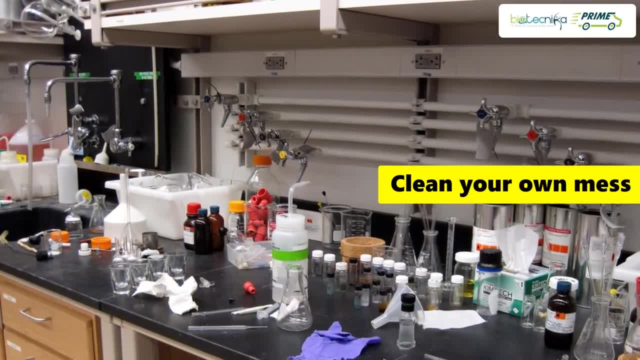 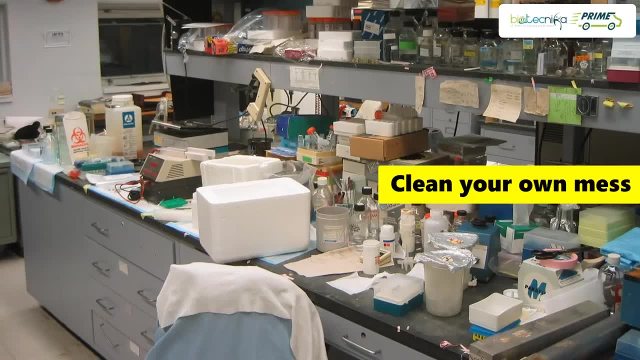 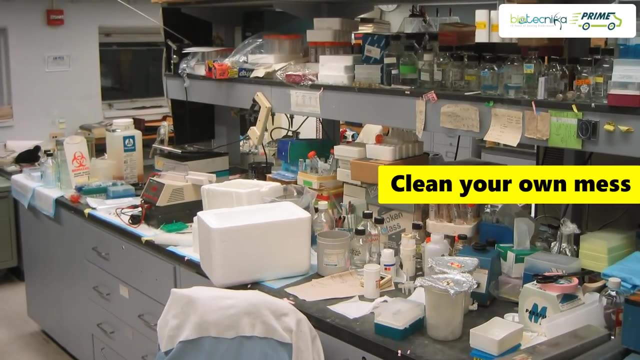 We may have many fellow researchers who tend to start their experiment, perform their experiment and end their experiments with some handsome results, but they just leave their mess for the other person clean. This is very harmful. Always make sure to dispose of the harmful lab waste carefully. 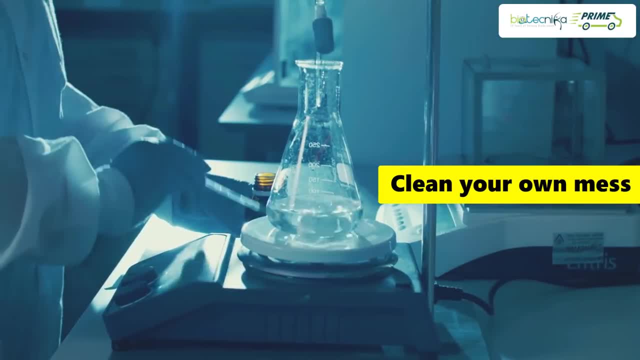 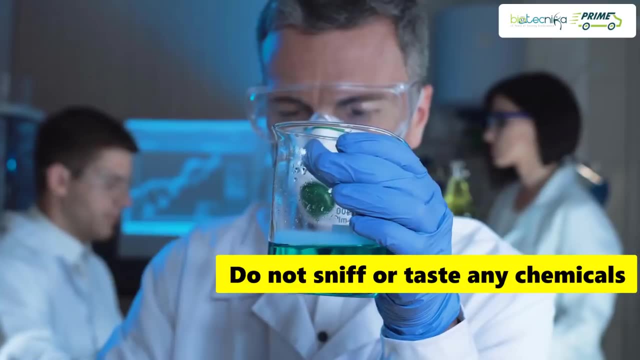 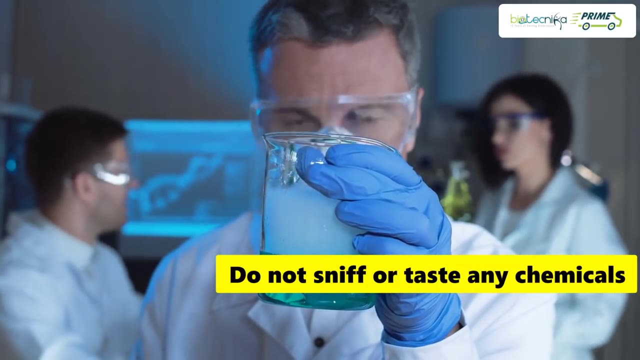 Because the other person may not know with which chemical or reagent you played Number 7.. Be Careful enough not to sniff or taste any chemicals. Many times people start pipetting by mouth. This is dangerous. Do not ever do this. 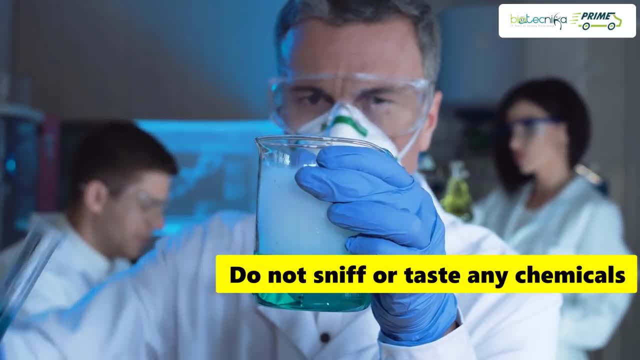 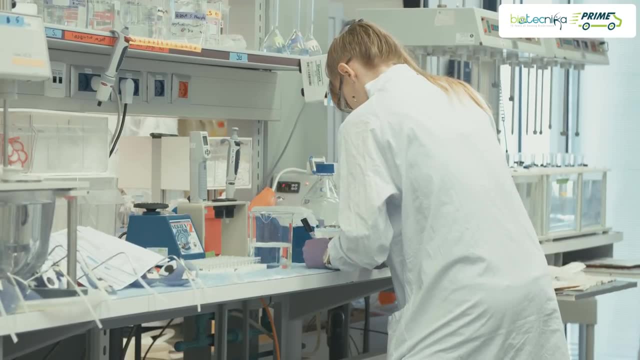 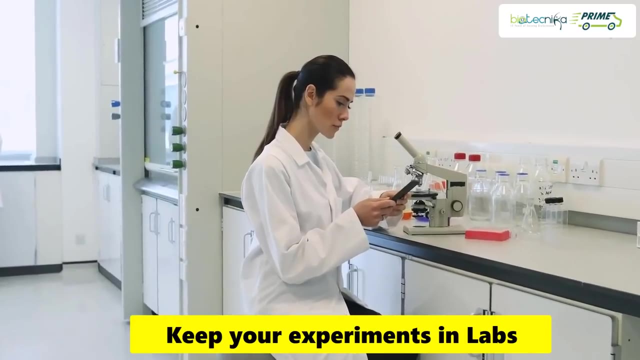 There are very high chances and risk of harmful and toxic chemicals getting inside your mouth. Number 8. Always keep your experiments in labs. You didn't have time in labs and it was late, but you are supposed to make cotton plugs, So you took them home along with a conical flask. 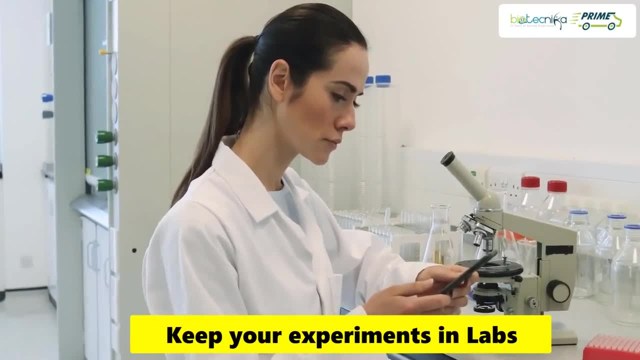 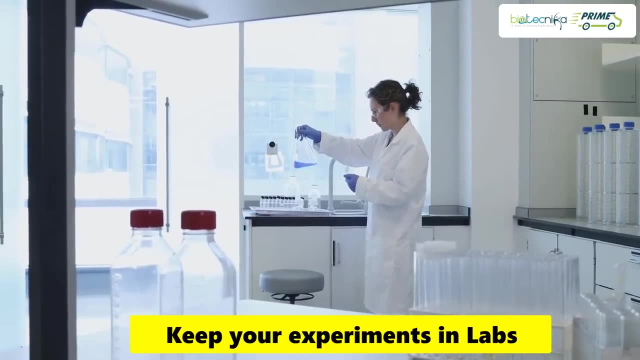 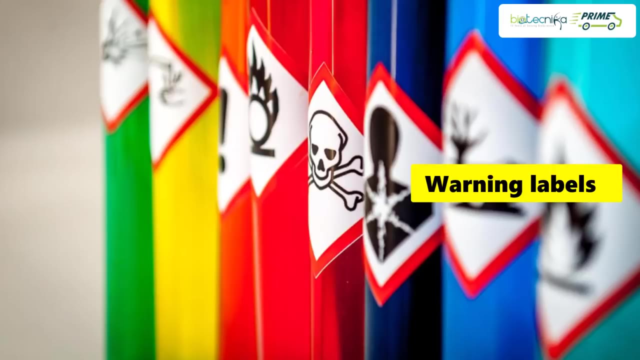 Do not take your experiments with you to your home or your other workplace as it may contaminate both your experiments and your outside lab environment, like of your homes. Also, avoid taking your lab coats outside the lab with you. Number 9. Do not undermine the warning labels. 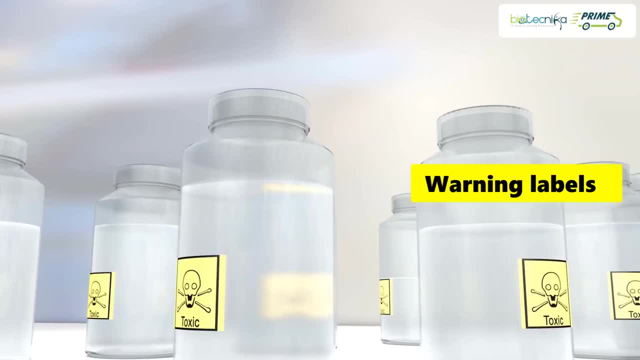 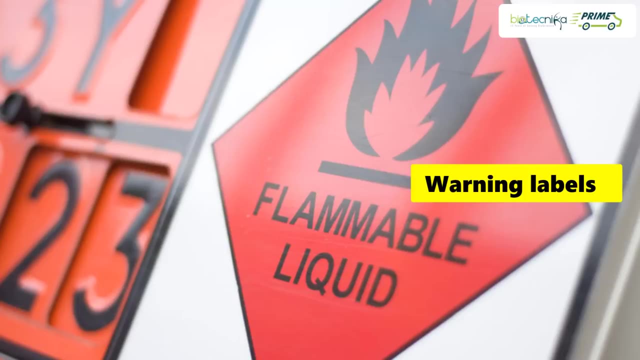 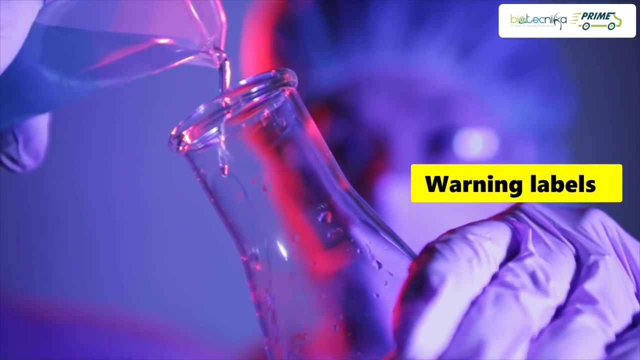 First of all, make a habit to use the important safety labels. Understand them and make others understand too. Store, Keep a flammable substance in a place which is fireproof. Be aware of the hazards and chemicals you are dealing with. Chemical mixing must be done carefully and not in front of your face. 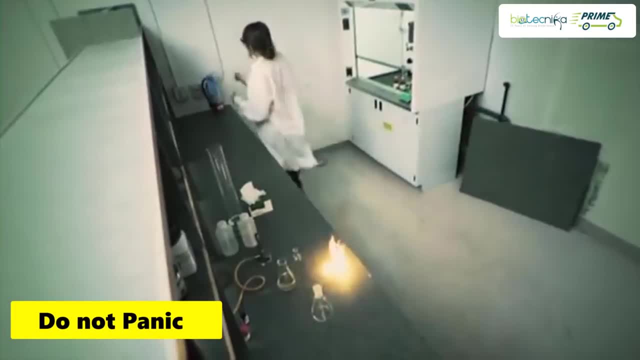 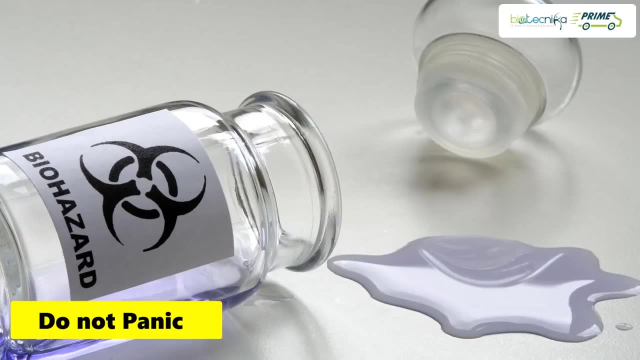 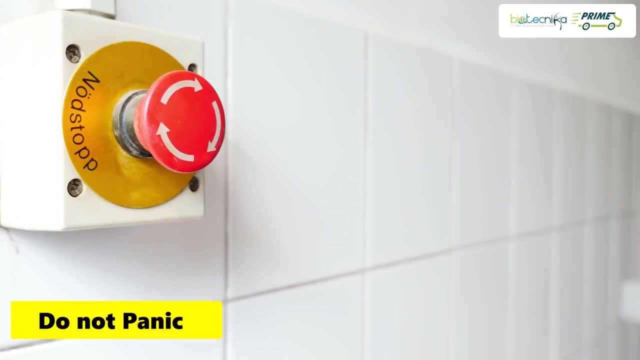 Number 10.. In case of any mishap, do not panic. Understand what can be done. in case of any casualty or an accident, Do not miss the lab safety drills and training which are given. Panicking only make things worse. Inform your supervisor or guidance. 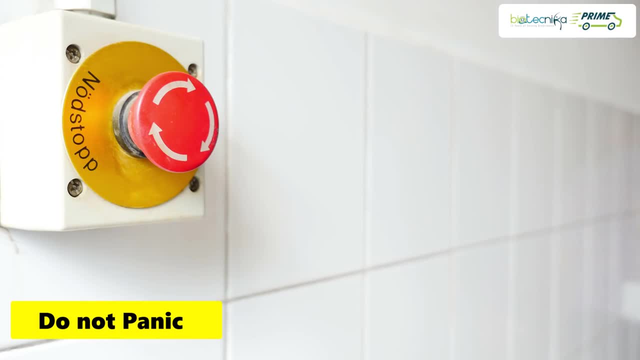 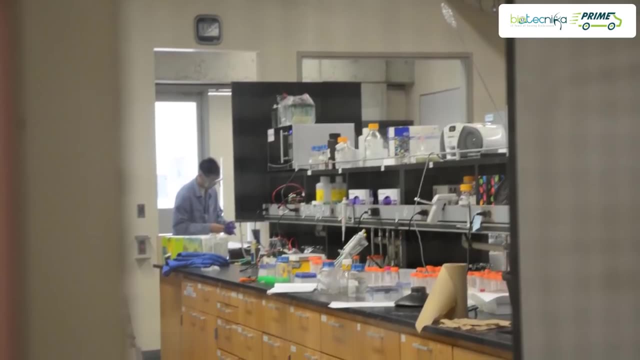 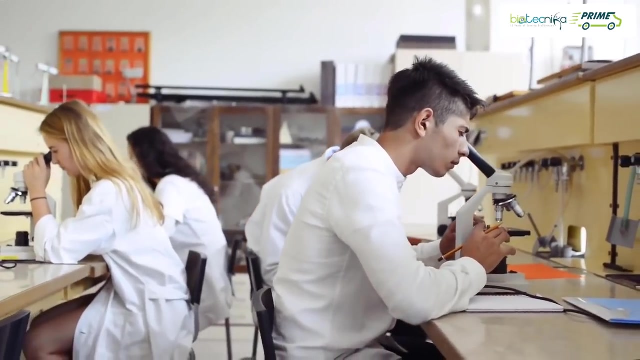 Do not be afraid about the experiment, but only with proper training and being careful you can avoid accidents. Accidents happen, but we can control it to every possible extent. Always mind it that it is not only you who are accountable. it is also about your research, mates or people around you. 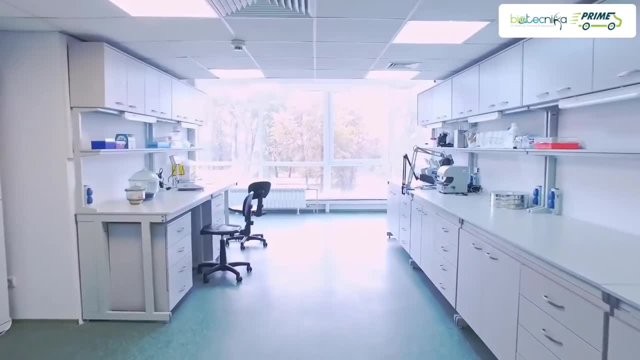 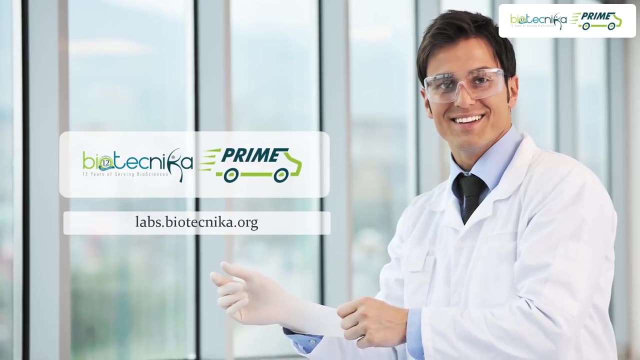 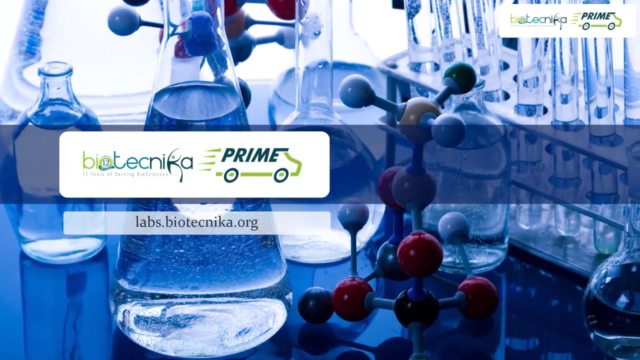 The danger will never be limited to you. Do not compromise on your research and your safety. Use the best and quality chemicals. We care for you At Biotechnica Prime. Be safe and be enlightened with Biotechnica Prime. Always buy certified chemicals and reagents.